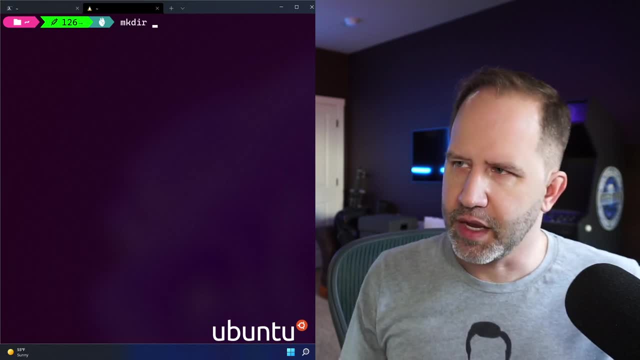 one makes you happy Doesn't matter. I'm going to go and make a My App folder and I'm going to go in there and you can see that it's empty. There's nothing going on here and I'm going to run. 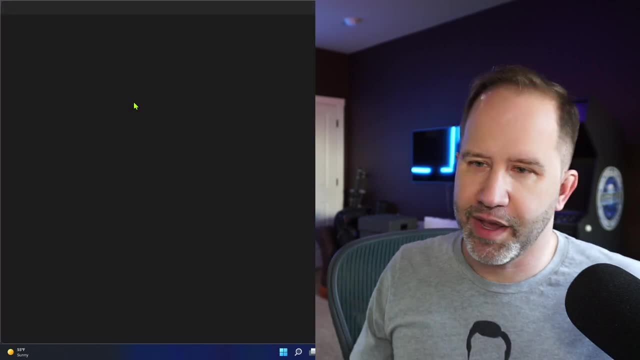 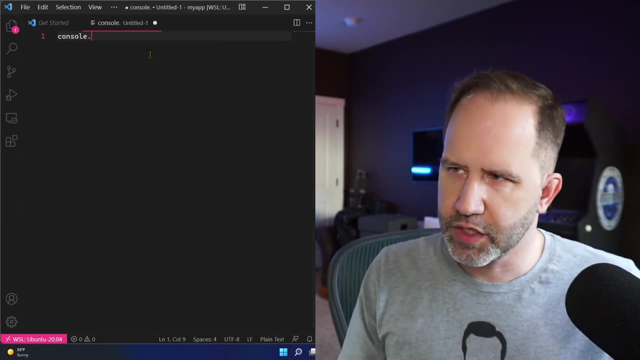 Visual Studio Code with code dot. I could run Notepad. I could run Microsoft Office. I could run Microsoft Office. I could run Microsoft Office. I could run something else, Doesn't matter, And then I'm going to say new file, I'm going to say console. 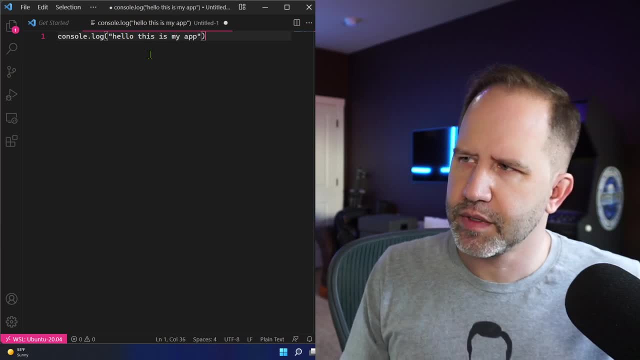 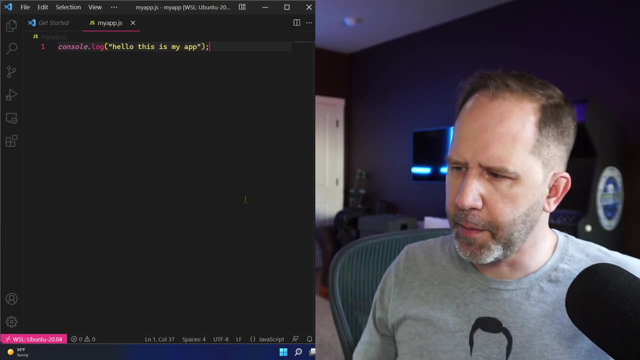 dot log. Hello, this is my app And then we're going to save this and we'll call it my app dot JS. We'll use JavaScript. You see, it just lit up there and Visual Studio decided that that has been auto-detected as JavaScript. I saved it as my app dot JS. We can come back here. We can look. 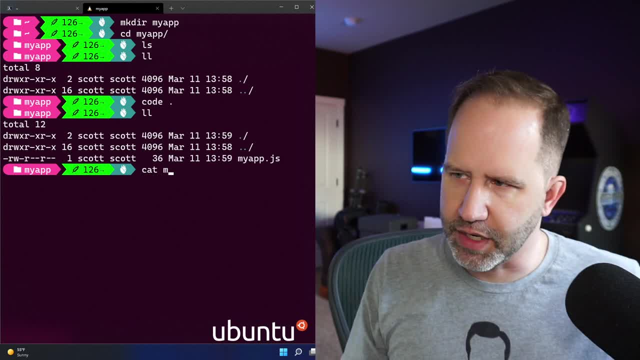 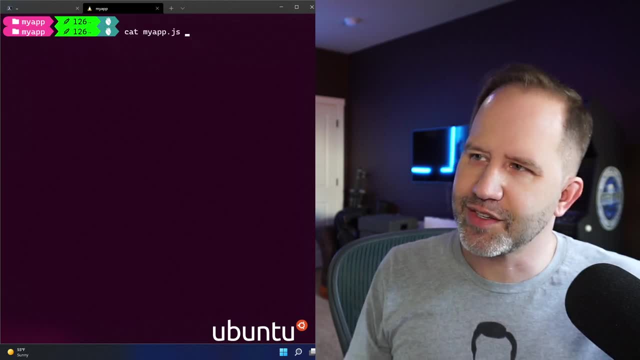 at our directory again. We see we have a little program called My App and I can look at it and it says console dot log. There we go And I'm going to say, actually, you see how it's when I do that, I end up getting my prompt right there again. That's because I didn't press enter. 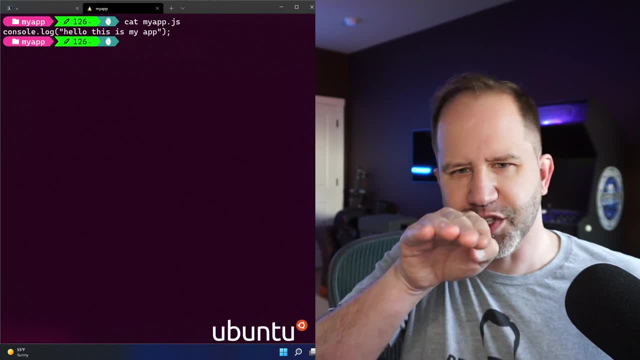 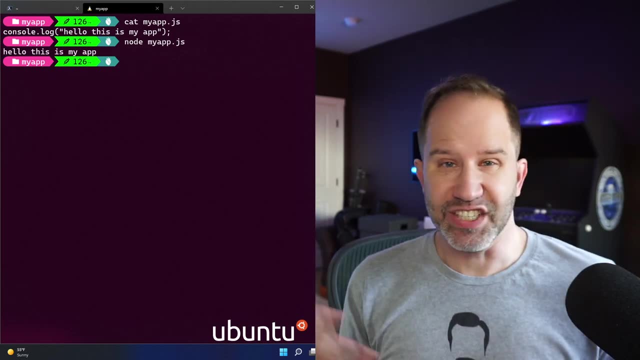 and then when I was outputting that, it didn't press enter on my prompt for me. so that's interesting. All right, I'm going to type node My App and it says: hello, this is my app. Is this on the client side of the server side? Well, 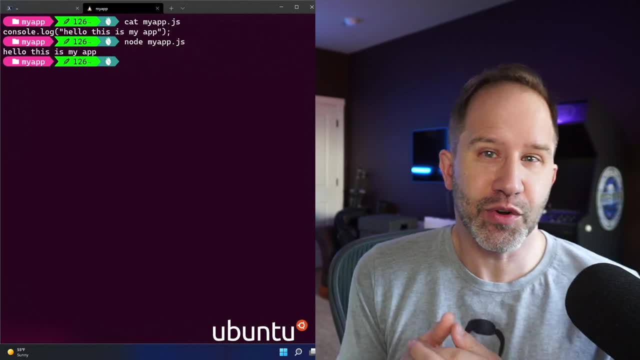 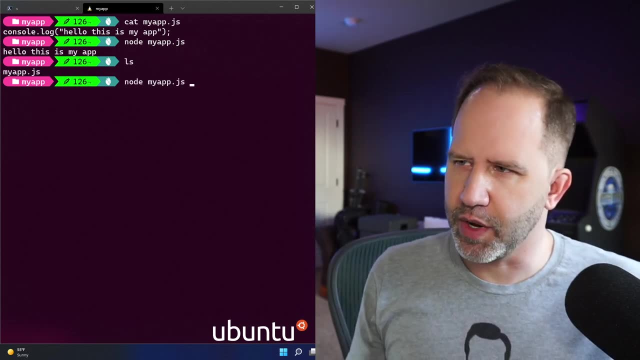 there is no client or server here, There's only my computer. My computer is arguably the client for a non-existent server. We're just running this app locally. It runs and it goes away. We ran it, It went, It's back, It's gone. Okay, That is JavaScript. 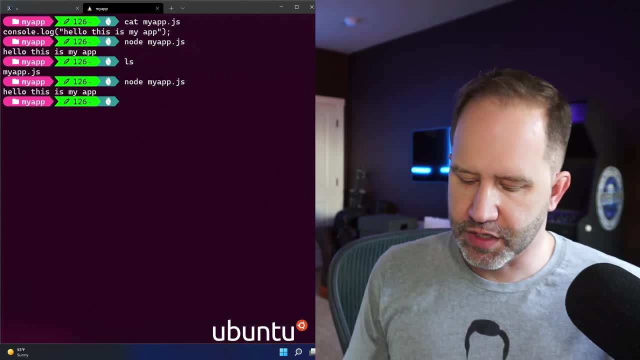 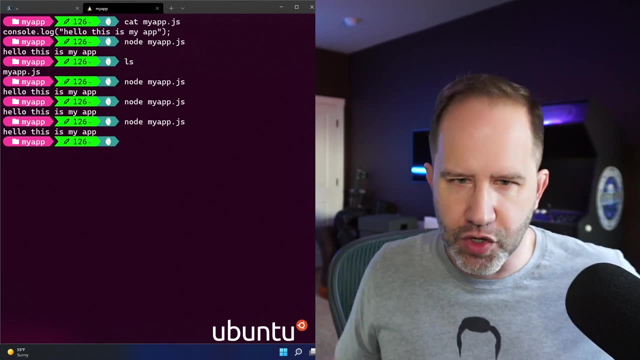 and it's running as a command line application. This is the command line or the prompt in my terminal here and that application ran and then it went away. So it ran within the context of node. Node knows how to speak JavaScript. It fires up this JavaScript engine and it. 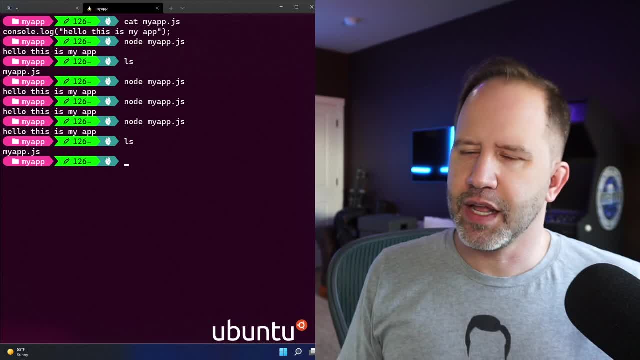 does the right thing When you run an application from the command line that doesn't have any connection. it doesn't have any connection. It doesn't have any connection to the application. It doesn't have any connection to the application. It doesn't have any connection to the application. 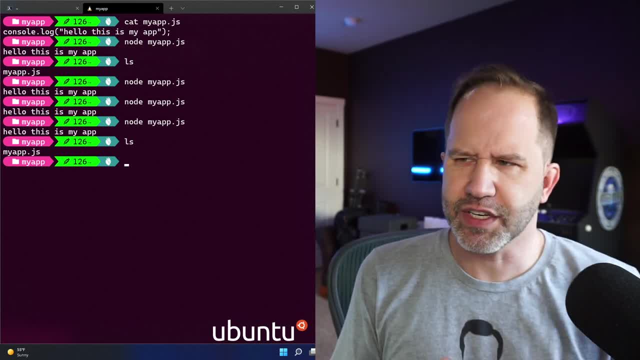 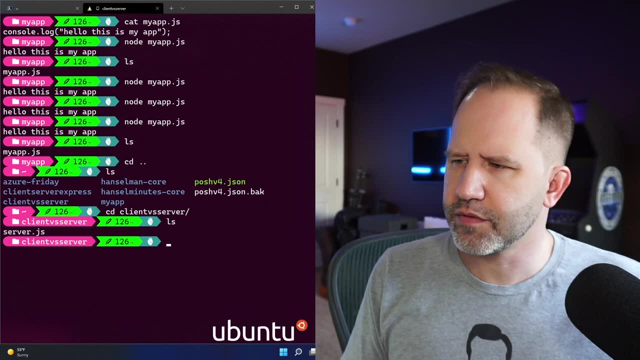 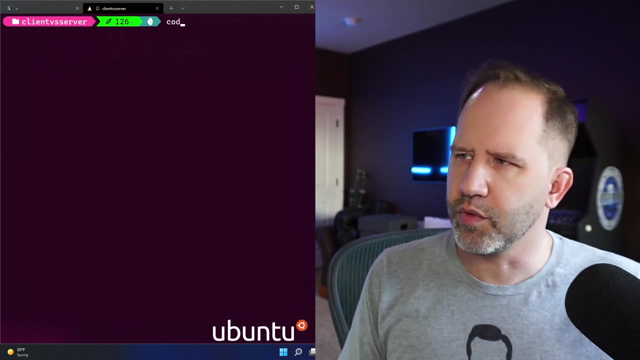 It doesn't have any connectivity to the outside world. that is entirely self-contained and running on my computer. However, let's go into another folder. Let's go to this folder here called client versus server, and in this folder I have a serverjs. Let's take a look, I'm going to run. 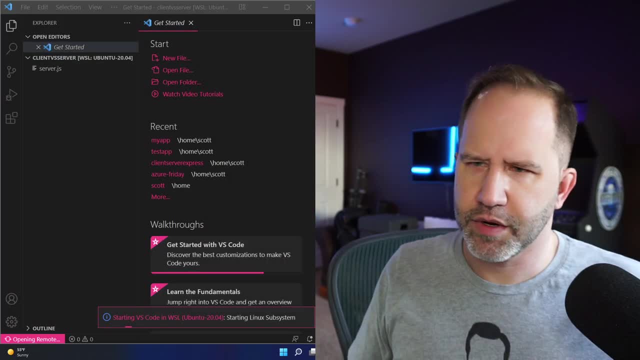 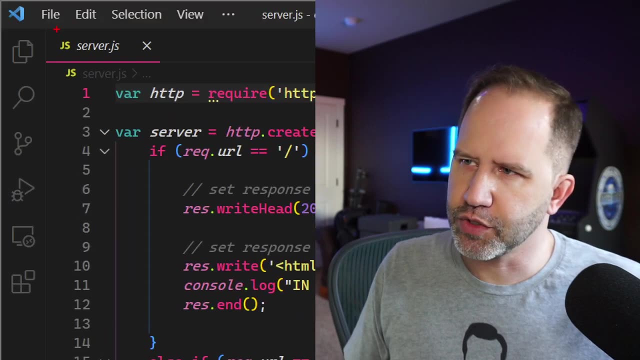 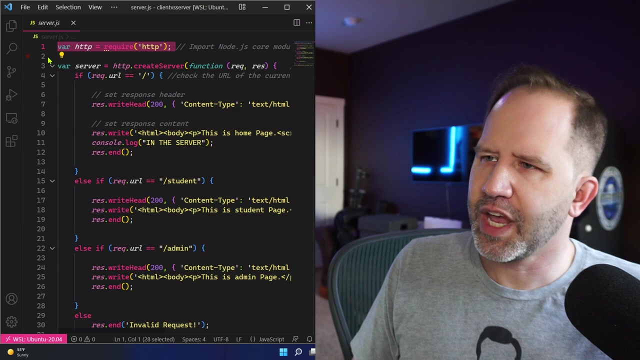 Visual Studio Code again. We'll bring this up here. and in here I have a serverjs. It doesn't And it's not called myappjs. And in here we say I'm going to use HTTP, the hypertext transfer. 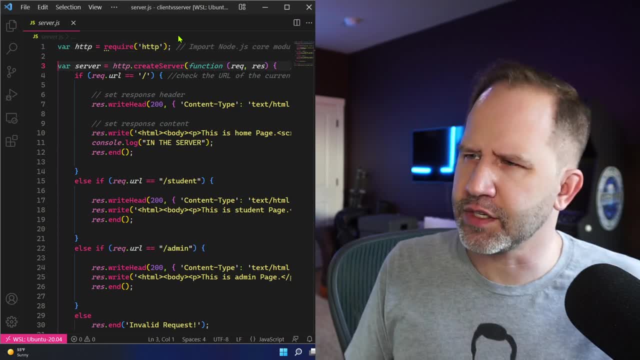 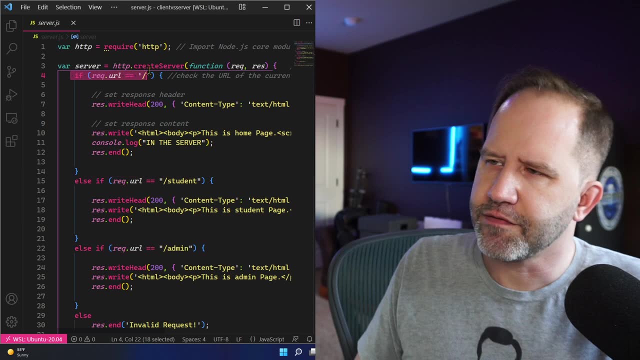 protocol and we're going to write a little server, a little server that a client's going to talk to. So we make our server and this is a little cheesy. but what we're going to do is we're going to say if the URL, if the address, has a backslash, it's only a backslash, or in this: 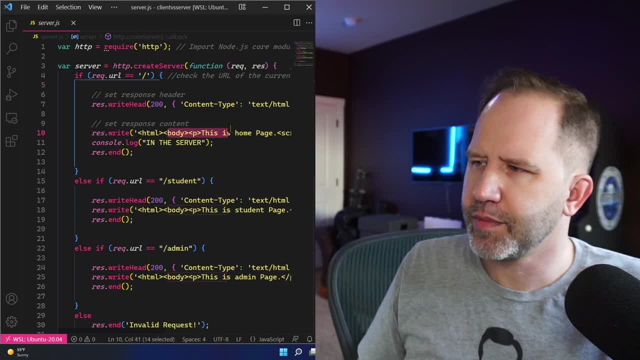 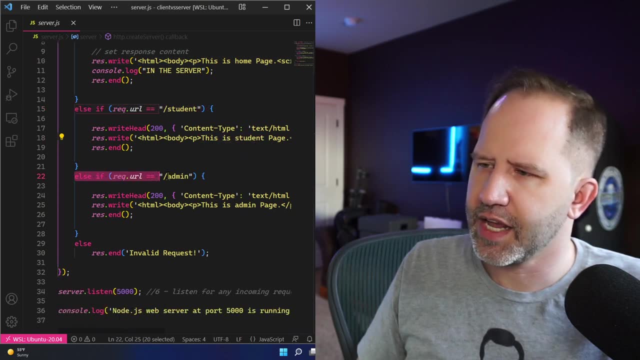 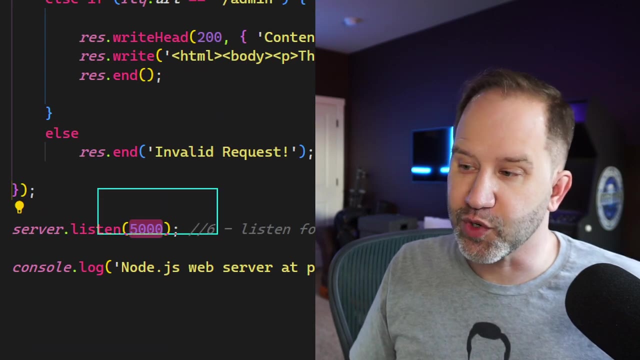 case a forward slash. we're going to output some HTML. We're going to say this is a homepage and then if you hit slash student, we're going to say this is the student page and if you hit slash admin, we'll say this is the admin page and we're going to listen on port 5000.. Ports are like: 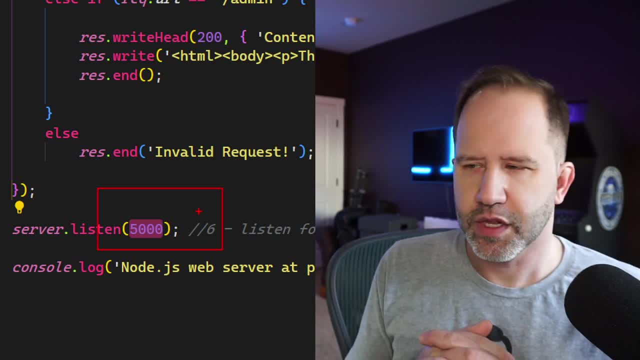 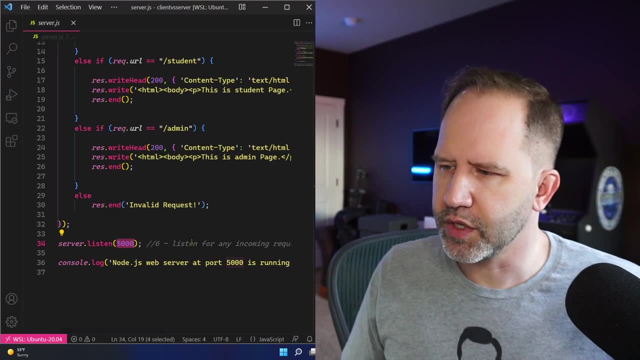 windows into your house. The computer is my house, The port is a window, so we're going to be peeking our head out of one window. The one we're going to listen on is 5000, and it's going to go ahead. 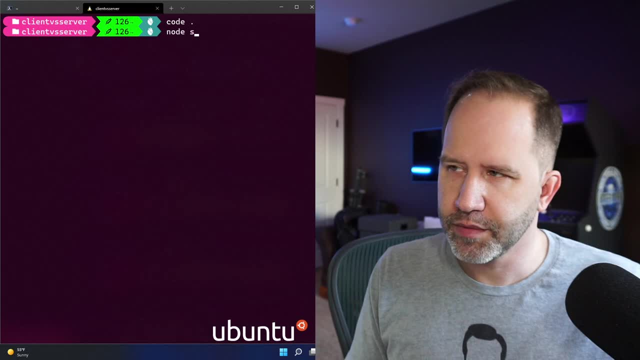 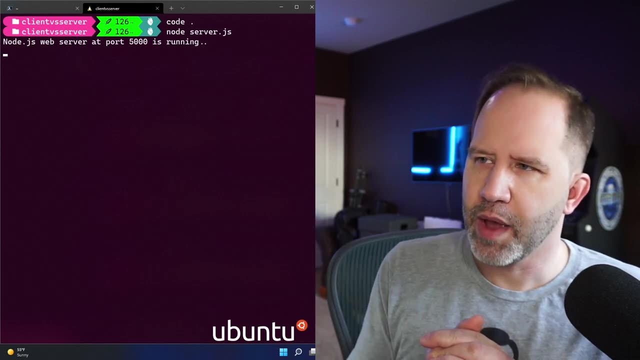 and start up. So what I'll do is I'll switch back over here and I'm going to say node serverjs, just like I said node myappjs. I ran the other one, I'm going to run this one, and here it says web server at port 5000 is. 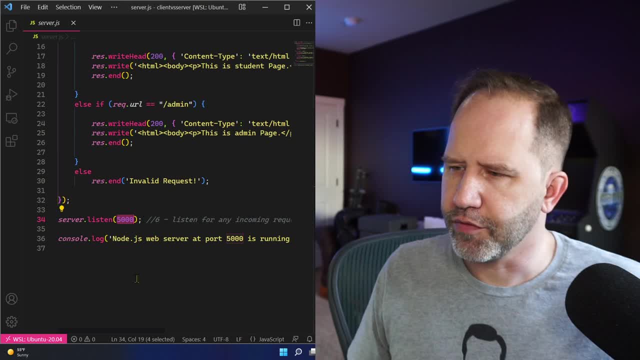 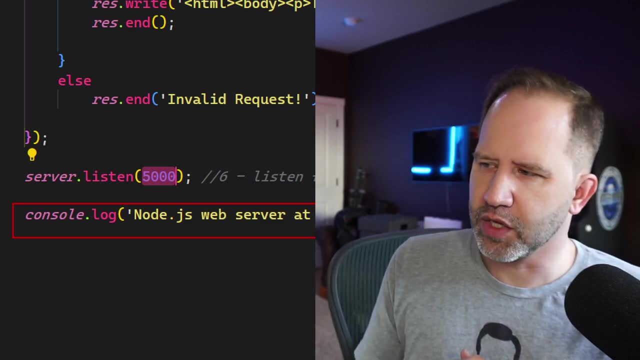 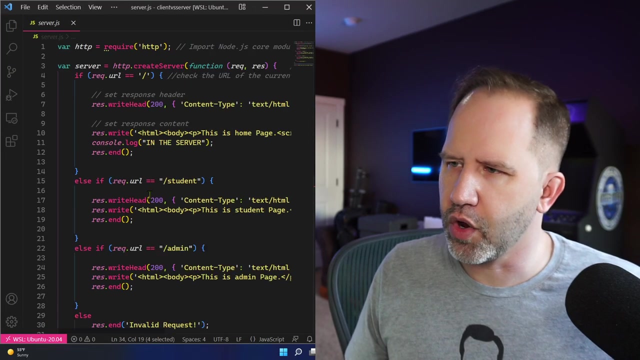 running. Now look at this. Remember before, when we said consolelog, we said: you know, hello, this is my app. Here I'm also saying consolelog and I'm outputting that we're running on this port, but then we have this other thing called server that's doing other work. All this other. 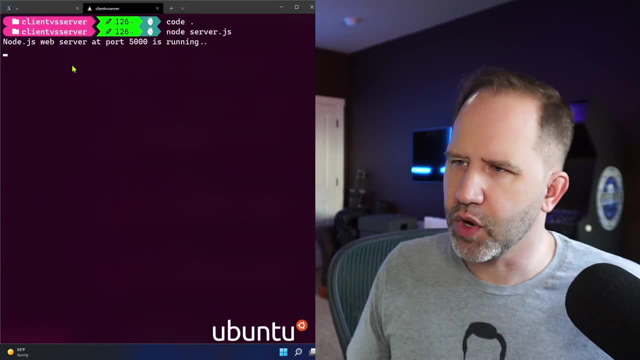 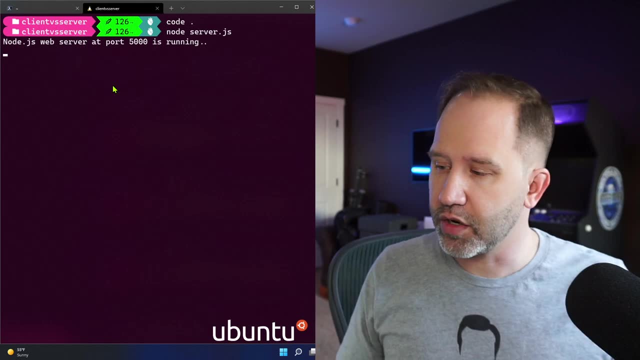 code. we didn't see any output there, did we? We only saw this. So that is running on my local machine and my app is running and it's listening. It's listening on port 5000.. Now I'm going to put myself in the corner here and we're going to bring up our 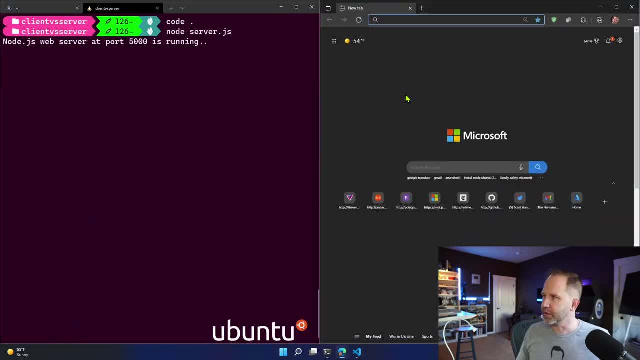 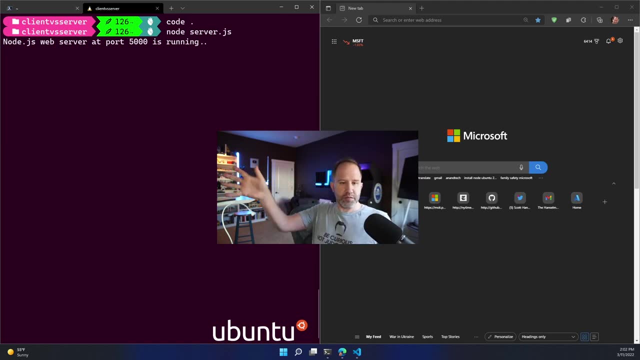 browser. We'll put our browser over on the right, okay. What I'll do actually is I'm going to put myself in the center here, okay? So here's our server. This is our server on this side and this is our client over on this side. They happen to be on the same computer, but pretend. 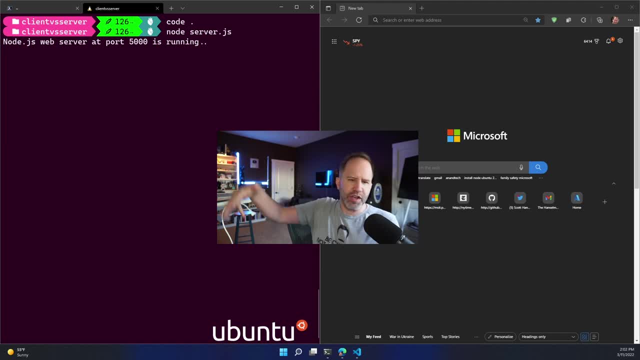 for a second that this is over here, This server that could be in the center here, That could be in Azure or that could be in Amazon, That could be some other computer somewhere else and over here, this is you. You're on your phone, You're on your computer, You're doing. 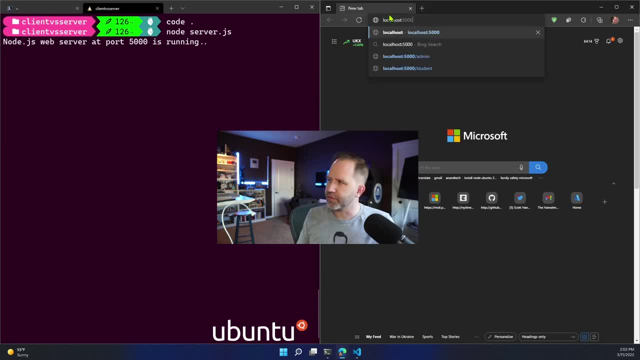 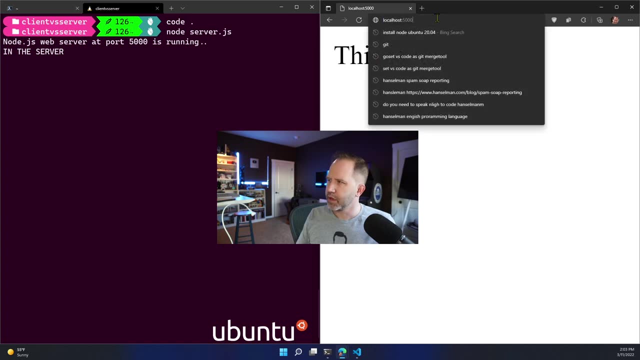 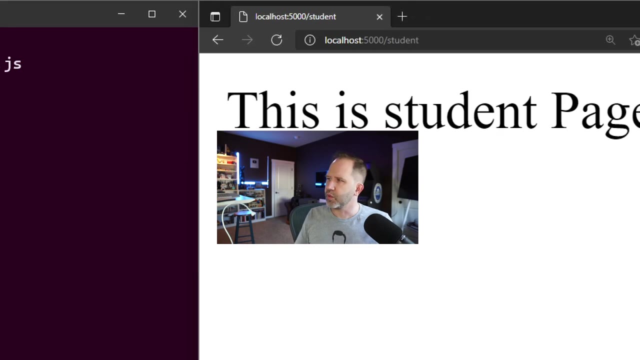 something and I'm going to type in localhost 5000 in the URL here and it says: this is the homepage. Cool, Let's hit slash: student, This is the student page. So we just on our client, on our client, up here our web server, we hit localhost 5000. 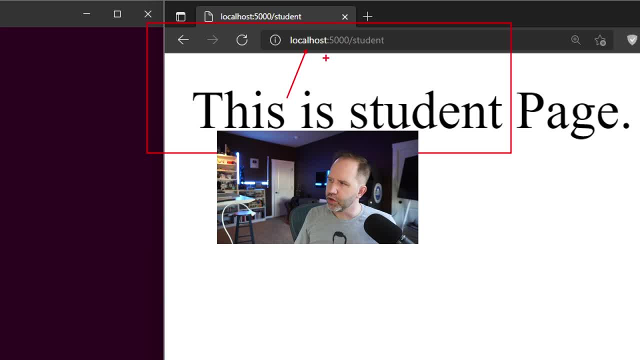 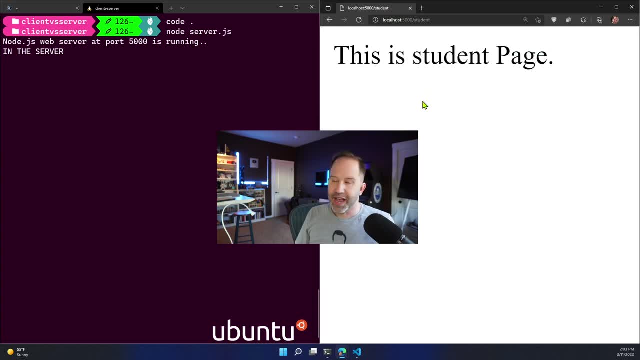 We hit localhost, which is my local computer, the machine I'm on here looking in that window, that port, port 5000, slash student, and we saw some HTML. We saw some HTML. I can actually move myself down over here and I'm going to right-click and say view source. 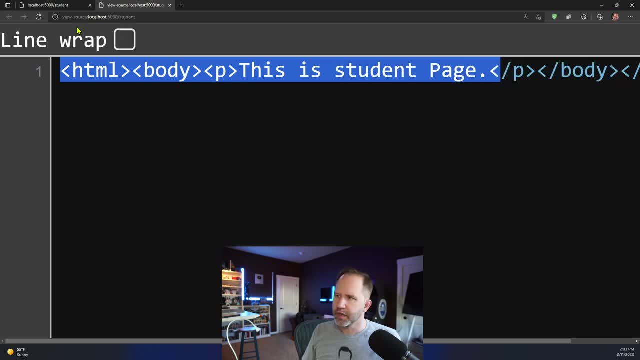 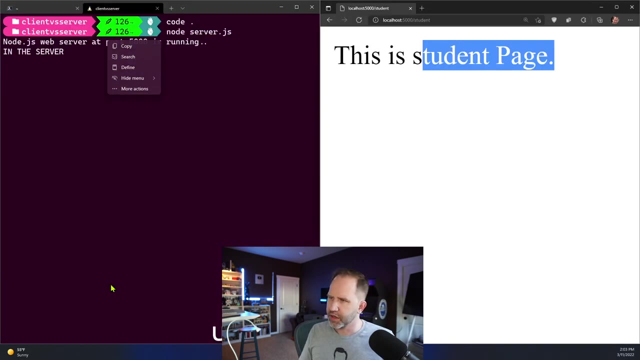 This is the student. We can actually see the HTML right there and we can see how it presented itself. So here's the source code for the web application. but this isn't JavaScript. This isn't JavaScript at all. There's no source code there. It's just how that was presented. but when we 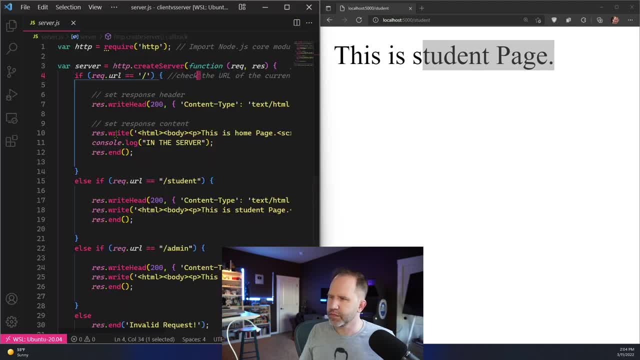 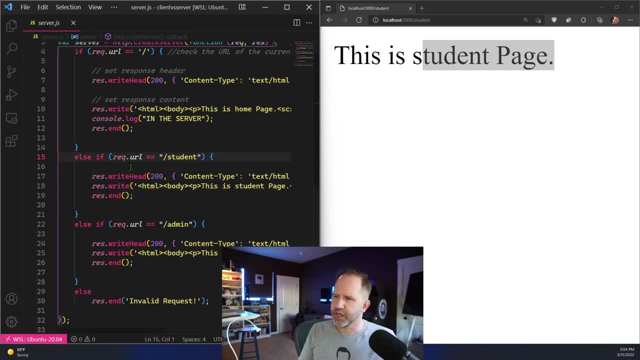 look over here in Visual Studio Code. okay, on the student page, we see that right there. Look, It says: if the URL is slash, student. we're going to output this as HTML and then we're going to write out to the response. We're going to write out to the response. this is the student page. 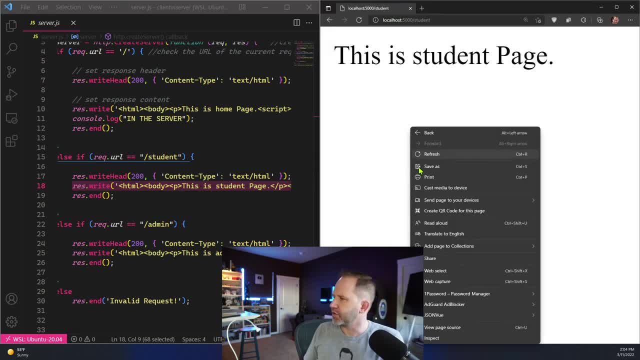 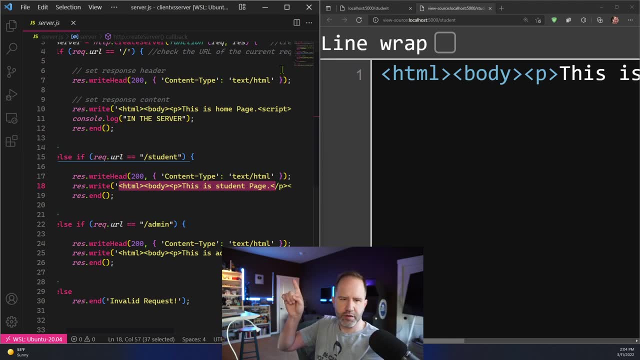 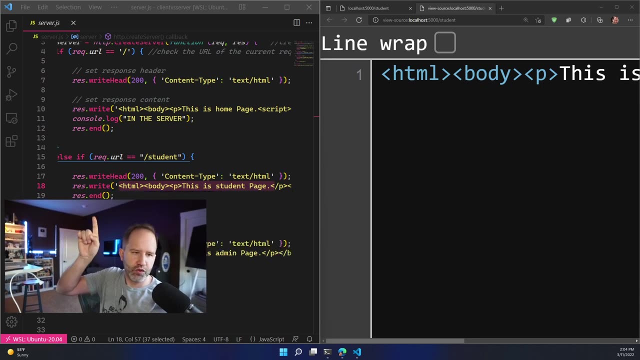 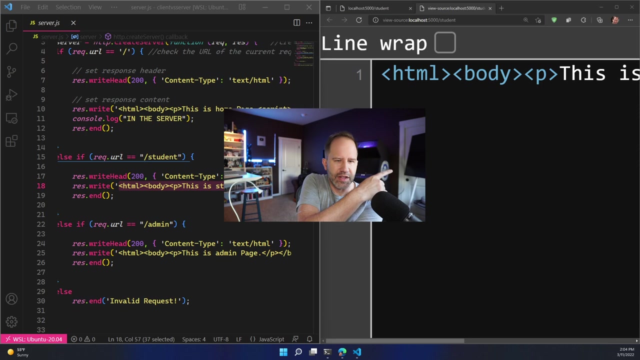 If I right-click over here and I say view source, this text right here, okay, this text right here, right here on the server was written out to the response and it got sent over to the client, right, and our client's over here now and that's how that string got there. 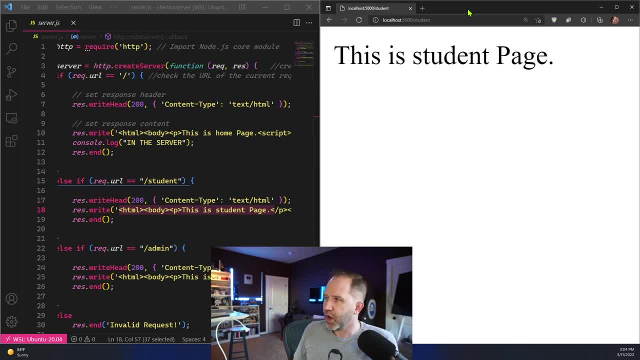 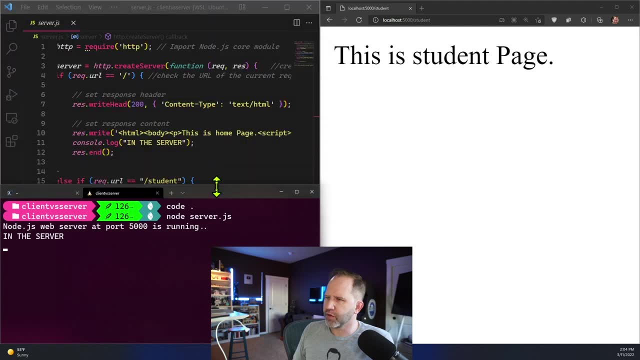 Now where things get confusing is: well, what code runs on the client, what code runs on the server? Let's take a look at this. This is a little complicated, but we're going to go through it together. Okay, I've added three windows now. 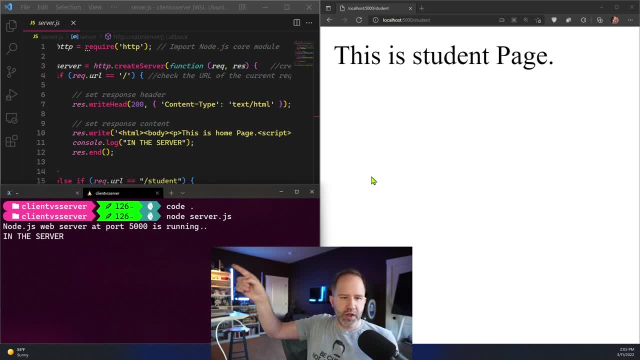 okay. So first we've got our little console app. that's kind of telling us what's happening. It's a console running on the server. Then we've got our source code up there inside of Visual Studio Code and then we've got our browser, our client over here on the right, and what we're. 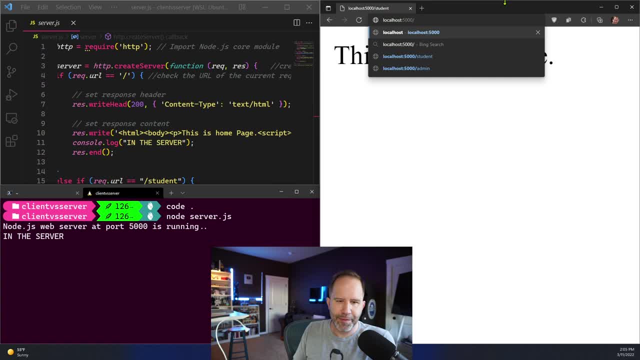 going to do is we're going to hit the home page here. I'm going to hit enter. so watch what happens Here when I press enter here. look at that. I'm going to hit refresh a bunch of times. I'm just. 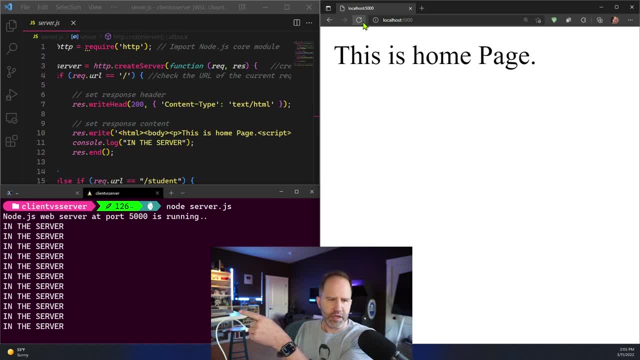 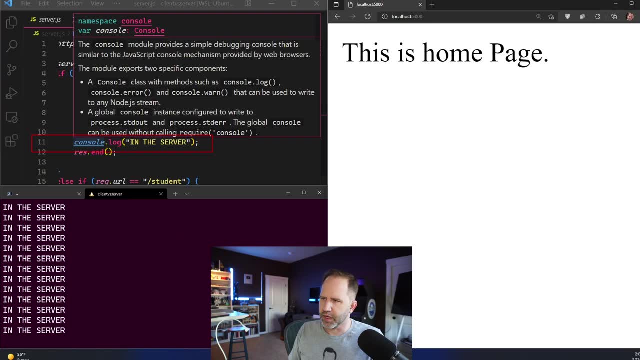 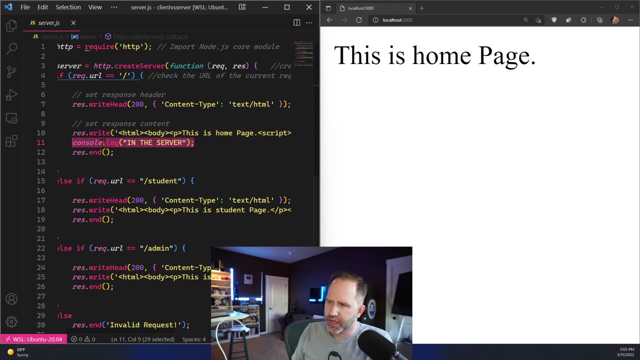 going to push the refresh button In the server, in the server, in the server. what's that? That line of code is this line of code? okay, So what we're doing is we're outputting this as the home page and outputting in the server at the exact same time. So we sent information. 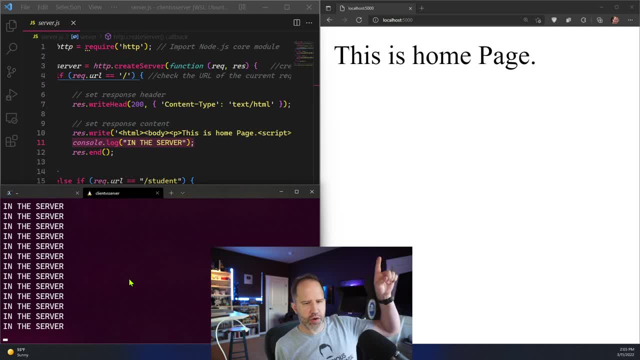 to our window here and we sent information to our client over here. So this way the programmers can look in the logs and see what's going on and they can debug things and they can say: I don't know, but mom and dad don't see that right, The clients don't see that, They only 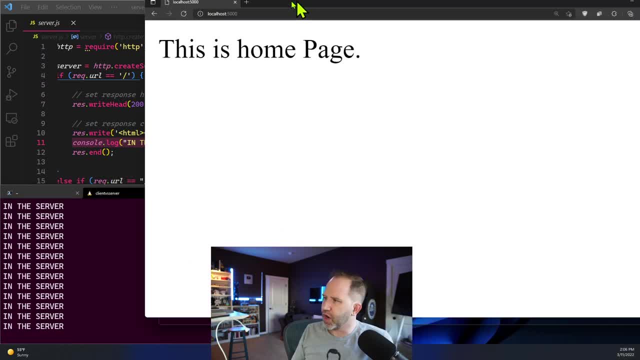 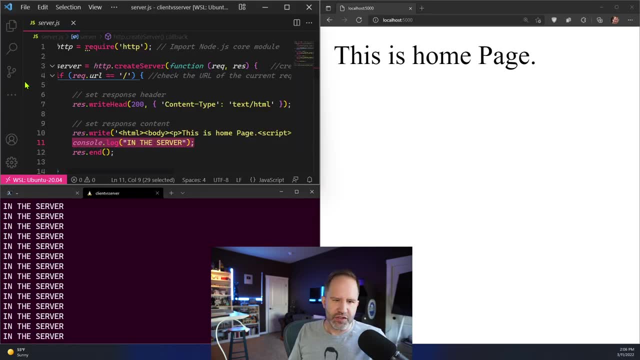 see what happens on the client side. So as a person browsing the web, I just see this. I'm just doing my thing. but on the back end, the back end is the server side. You hear about the front end, the client, and the back end, the server. 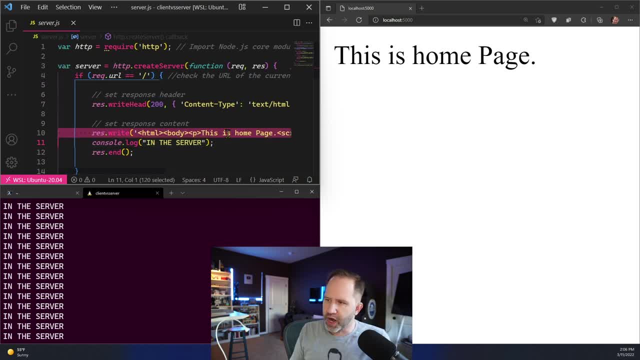 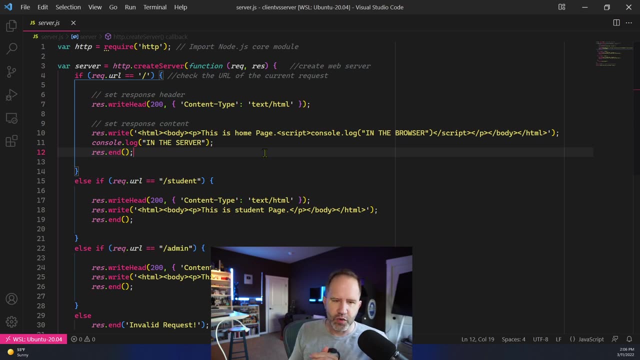 On the back end there's things happening. We're writing out to the response and we are saying, for logging purposes, hey, we're on the server. Now here's where things get squishy. He said, yeah, but I need to write JavaScript on the client side. I need to do client side JavaScript. 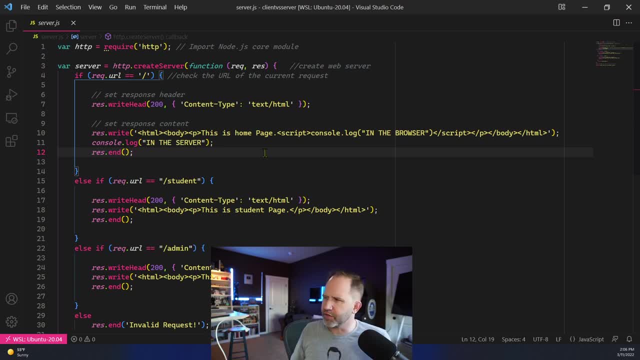 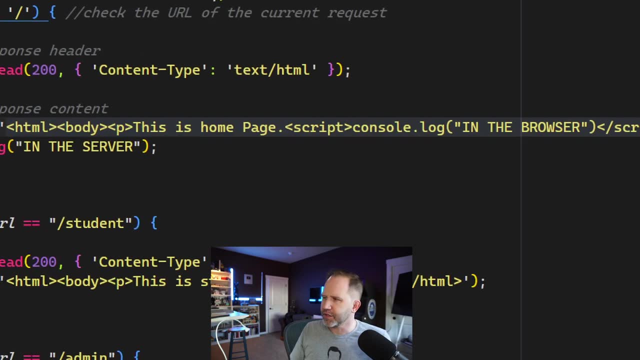 but I just wrote this whole thing. that is server side JavaScript. So what I've done here is something you shouldn't do. This is not good, but I'm just showing you this for educational purposes. Notice this line 10 right here. okay, We've got this as the home page and I've got some inline. 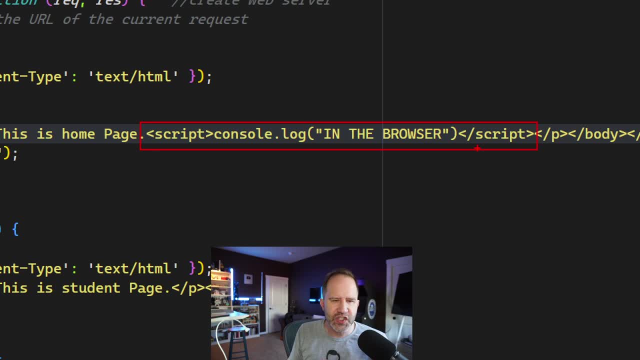 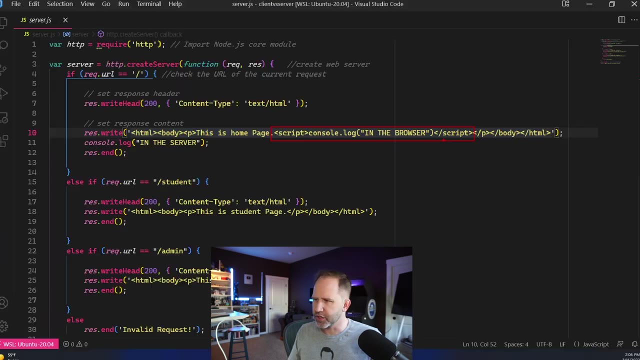 script. So I'm going to send some JavaScript, along with my HTML, over to the browser. over to the browser, and that script is going to run. Now. we've seen consolelog before. We saw consolelog just a minute ago, right, Consolelog saying, hey, I'm on the server, but this consolelog is going. 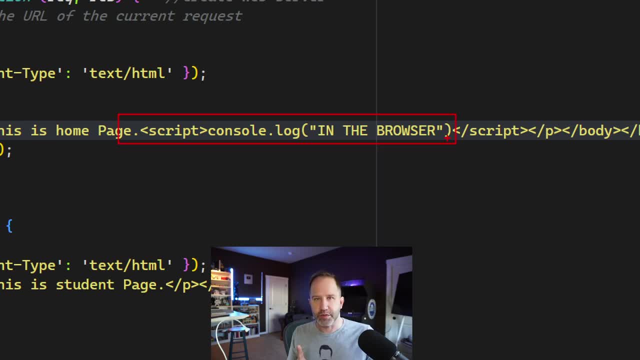 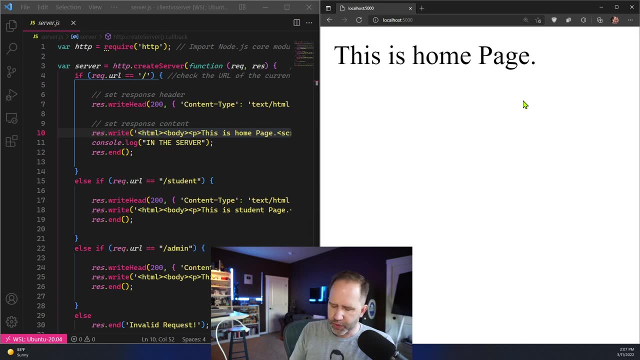 to say: hey, I'm in the server, So I'm going to send some JavaScript, along with my HTML, over to the browser. They're both JavaScript. They're both JavaScript, but browsers come understanding JavaScript out of the box. So what we're going to do is we're going to press F12, the F12 button. 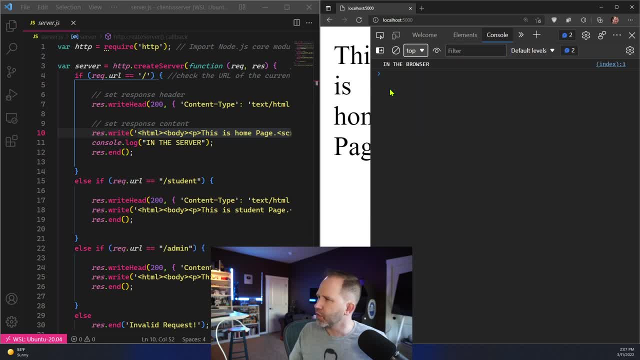 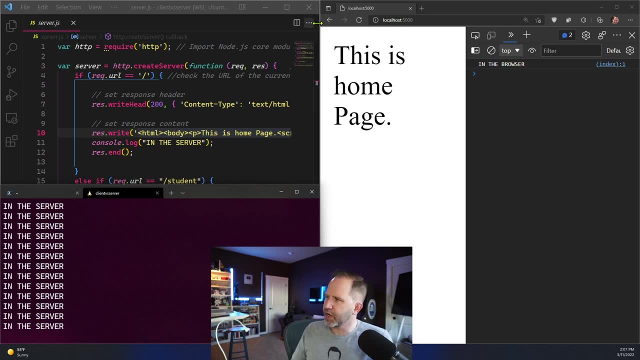 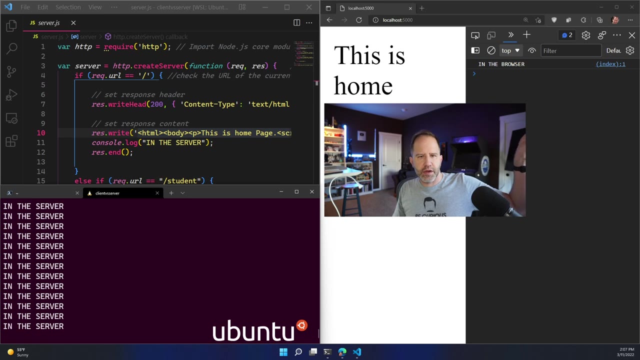 okay, We're going to press F12, and what I'm going to do is go like this and go like that, and then we're going to hit refresh. So you're going to watch on the server here and then you're going to see in the browser right here. 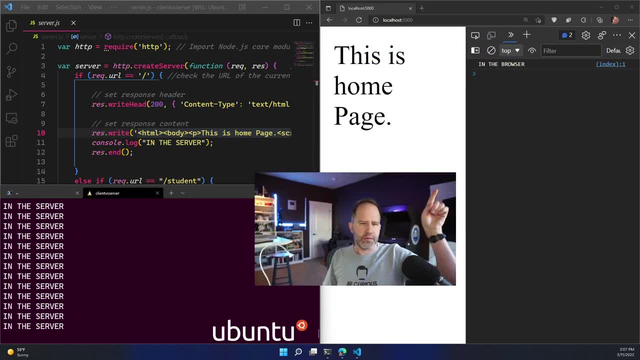 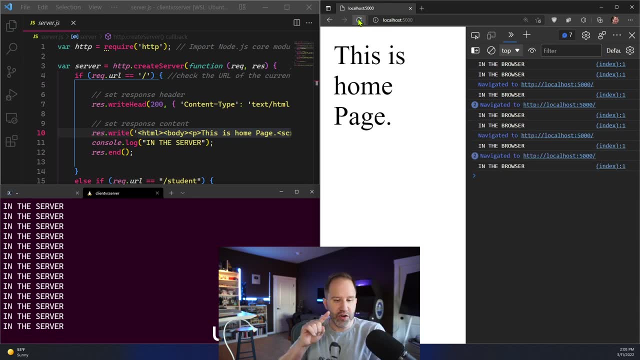 There you go. Okay, Hit refresh. So each time I'm hitting refresh the server listens on that port 5000, runs its code. It runs this consolelog in the server. It sends that response over to the client, sends that response over to the client. The client then receives the HTML and says: 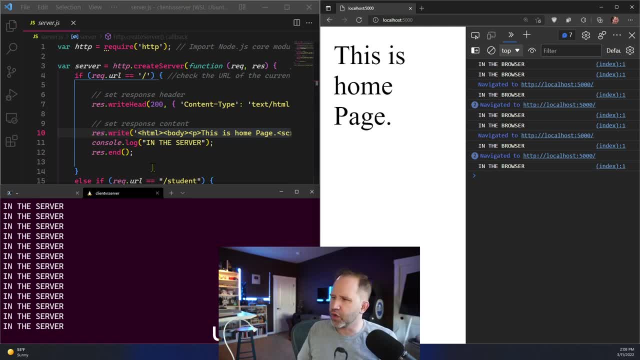 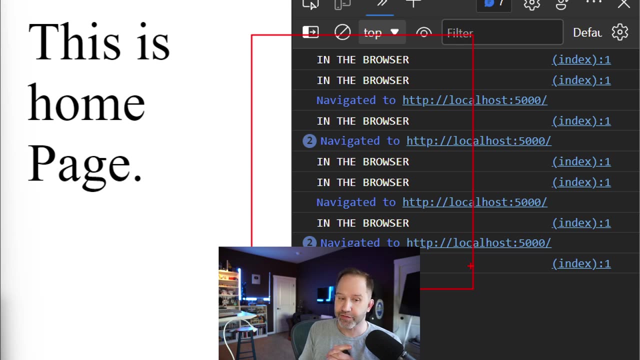 this is the homepage. Inside of that HTML is also: we saw some embedded JavaScript. We sent some JavaScript along for the ride and that said in the console. the console that we got from our dev tools or our F12 tools, said in the: 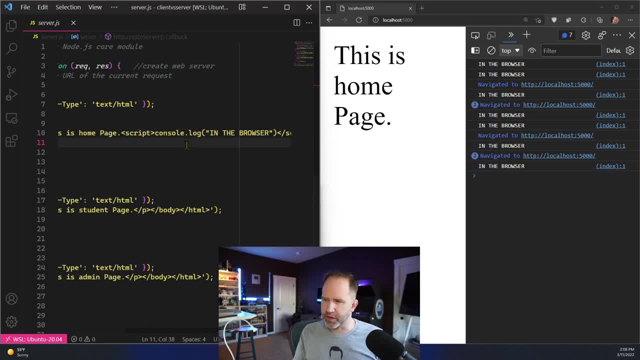 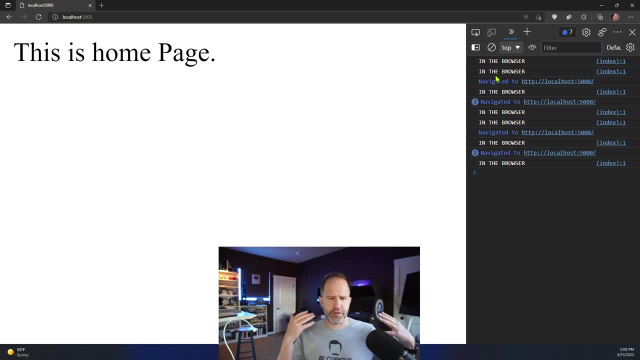 browser in the browser. So in this case we have JavaScript on the server and JavaScript on the client. but if we remember that the person on the front end, the user, non-technical parent, they're experiencing JavaScript, So we're going to hit refresh. So we're going to hit refresh. 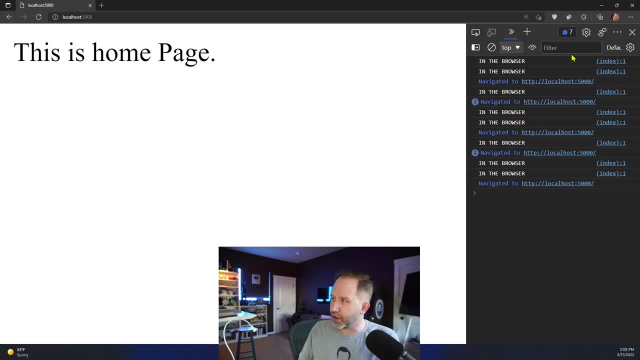 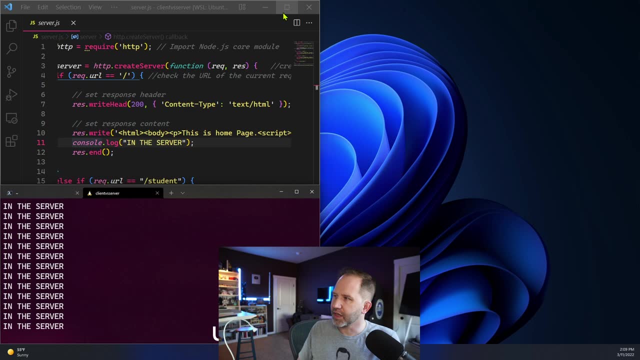 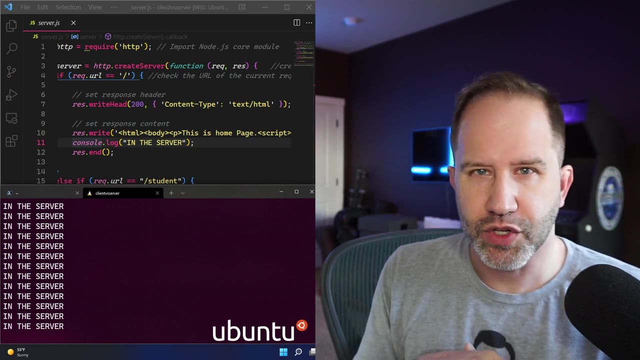 You'll notice that they're just saying this. they probably won't ever even see this consolelog Here. that can be debugging for you, the developer, but that's an interesting way to think about the client and the server. Okay, If you like beginner videos like this, let me know in the chat what you. 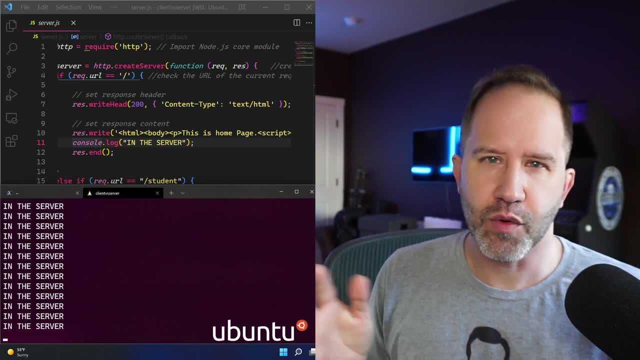 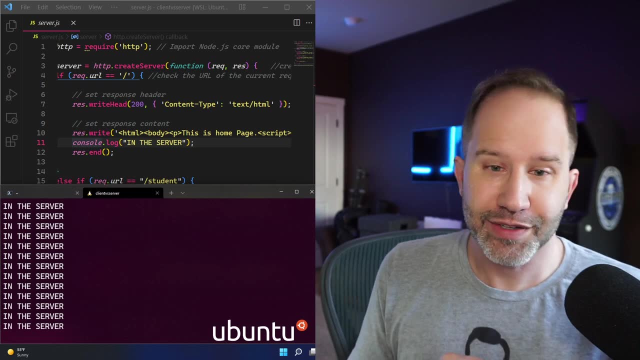 think we should talk about in the future. I do realize that for some of you this is very 101 beginner-level content, but this was a question that my nephew had And now I wanted to put it out there on the internet because apparently they didn't teach it in school and I wanted to let you know.